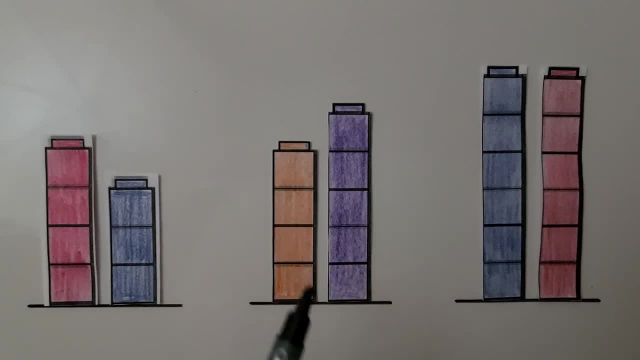 We have a set here. We have a set here and we have a set here. When cube towers are the same height, they will have the same number of cubes and they will end in the same place. We need to circle the set of cube towers that are about the same height. 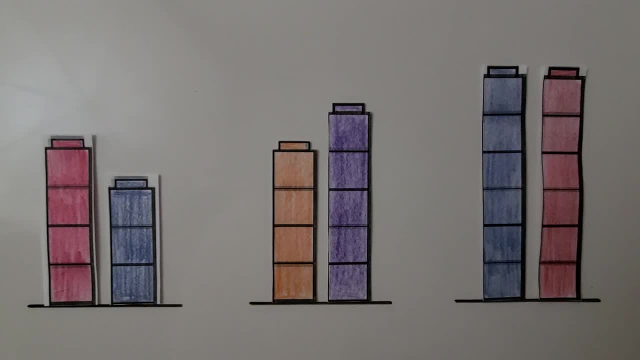 Can you tell which set of cube towers are about the same height? Is it this set? Is it this set Or is it this set? If you said this set, you're right. we need to circle this. That is the set of cube towers that is about the same height. 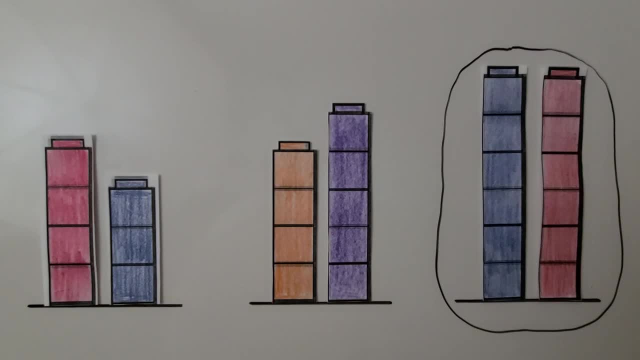 When a cube tower is shorter than another cube tower, it will have fewer cubes and not be as tall. The blue cube tower is not as tall as the red cube tower and it has fewer cubes. This one has one, two, three, four, five, six, seven, eight. 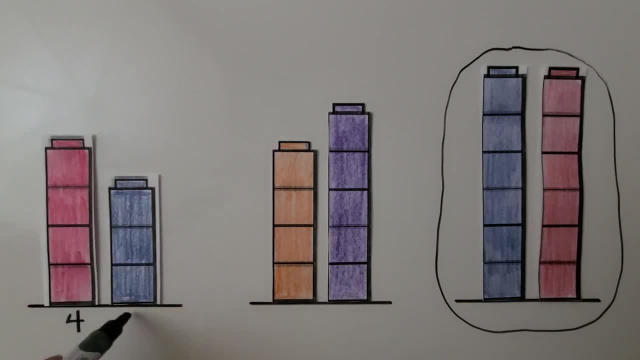 I got two, three, four, five. I got two, three, four, five. This one has one, two, three, four cubes. This one has one, two, three cubes. It has fewer cubes When a cube tower is taller than. 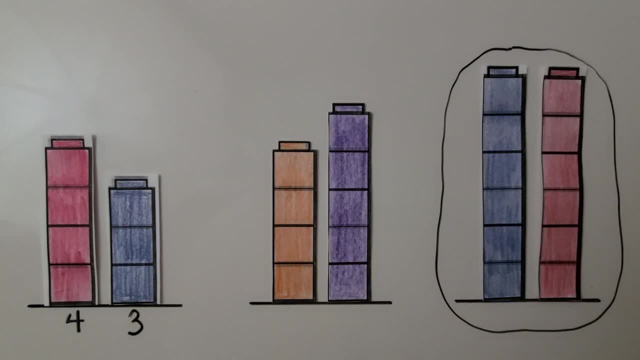 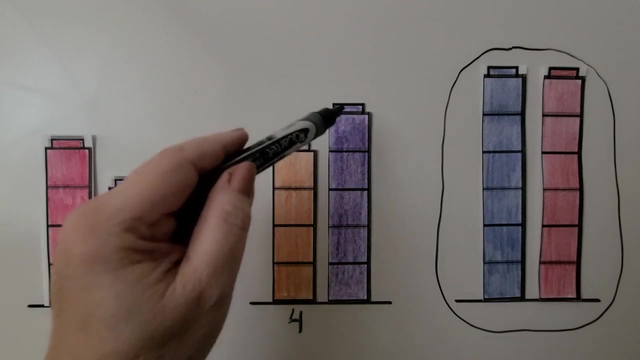 another cube tower. it will have a greater number of cubes and go up farther. The purple cube tower is taller than the orange one. It goes up farther than the orange one And the orange cube tower has one, two, three, four cubes And the purple cube tower has one, two, three, four, five cubes It has 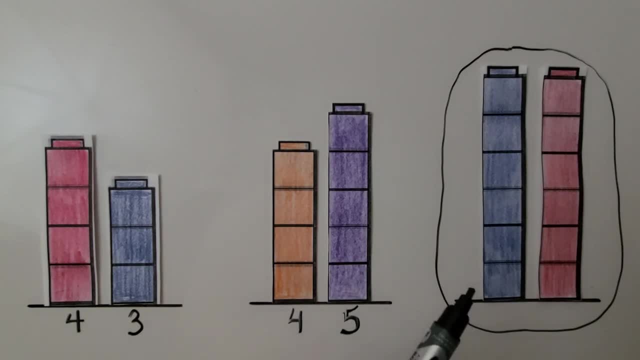 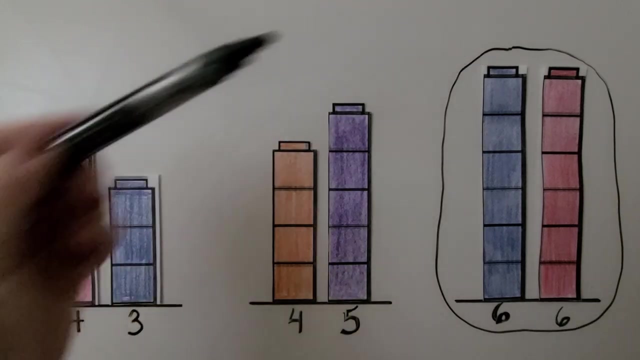 more cubes For our set that has about the same height. the blue cube tower has one, two, three, four, five, six cubes And the red cube tower has one, two, three, four, five, six cubes. they have the same number of cubes and they're about the same height. 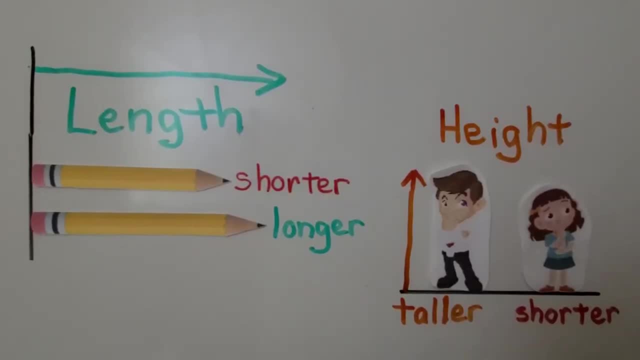 So remember that length is different than height. Length tells us how long something is and height tells us how tall something is. Our next lesson, 11.3, we're going to do some problem solving and direct comparisons. I hope you'll join me. I hope you have a wonderful day. and I really hope you'll hit the like button. Bye.